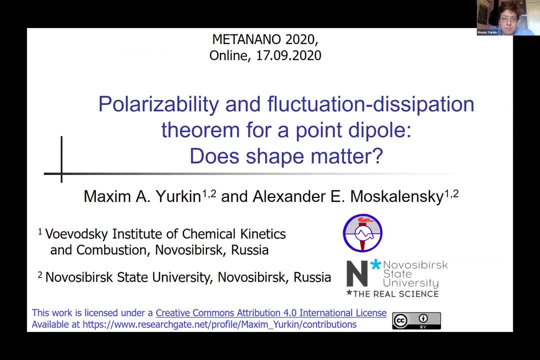 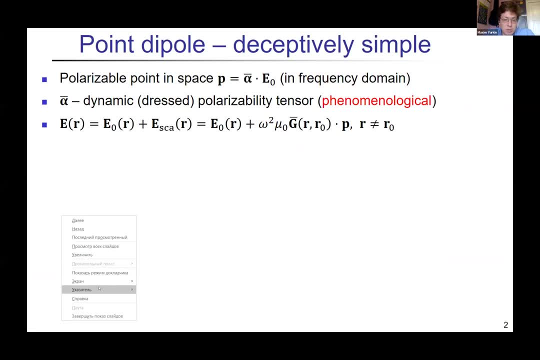 So yeah, I will be talking about point-dipole and fluctuation, dissipation theorem, And the concept of point-dipole is, I mean, everybody knows what is it. It's really simple, but I would argue it's somewhat deceptively simple. So I will be talking only about frequency. 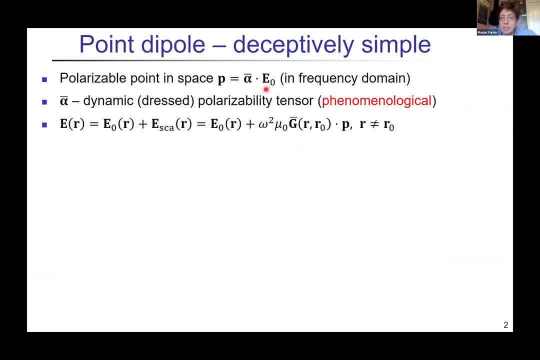 domain. Then you have incident fields like inot, and the dipole moment is related linearly to it and I will everywhere use dyadic or tensor. so for general description, And in this description it's really a phenomenological constant. so the frequency is fixed And once 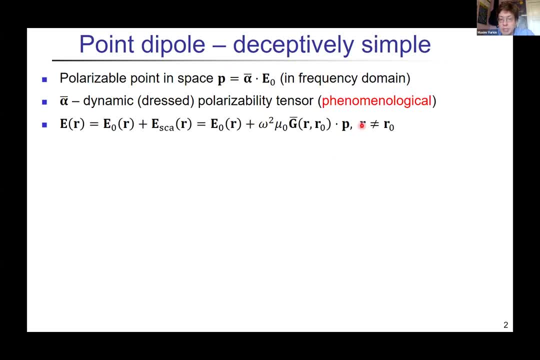 you fix this, then you also have field everywhere in space given by this quantity, where G is the green stanza, either of free space, which is trivial, or some environment that is present like substrate near the dipole. So that's all known. but then you want some other measurable. 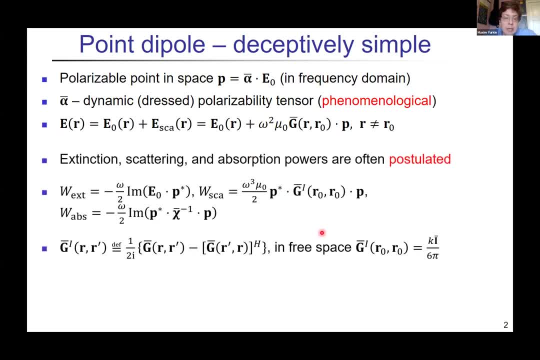 quantities Like extinction, scattering and absorption powers. And here again some confusion starts in the literature that sometimes they're derived, sometimes they're postulated, and here are some of the possible expressions for that So important part: that for scattering here we use the GI. 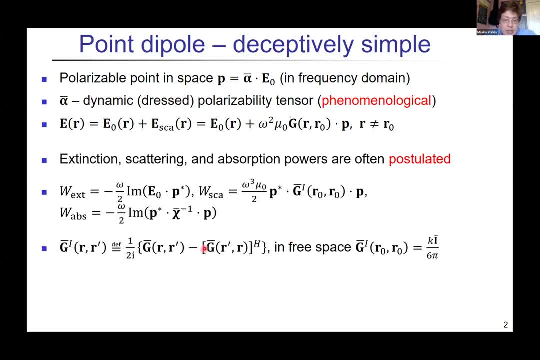 which is kind of imaginary part of the green stanza, but more generally it's Q Hermitian part. So in free space it's just basically unit dyadic, But in some environments it can be more complex, And also in this phenomenological description. 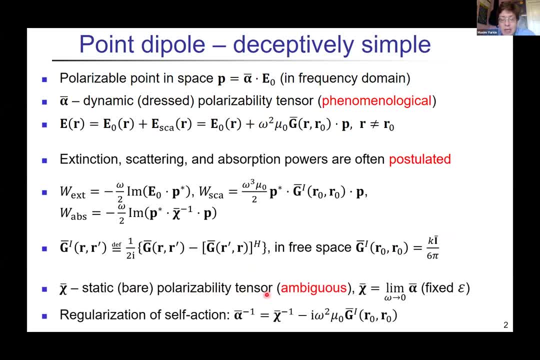 we don't have chi, so static or the bit of tensor. Again, there is a confusion with name in a lot, so I will use static, or it's called pair plausibility And alpha is like dynamic or trace plausibility tensor. 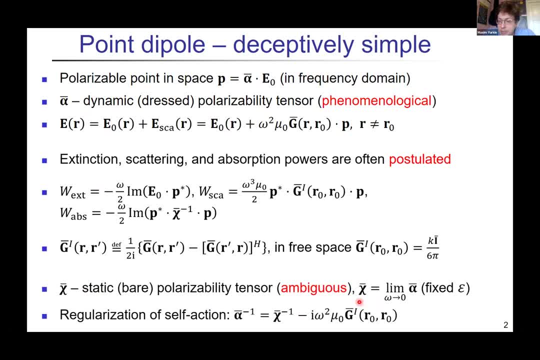 But the problem is that. so you can. you can write some definition like that that chi is a limit to zero frequency, Okay, But it's not really operational unless you have some microscopic model, because in phenomenological model that we discussed here, well, for now it's just a constant, so you can't really. 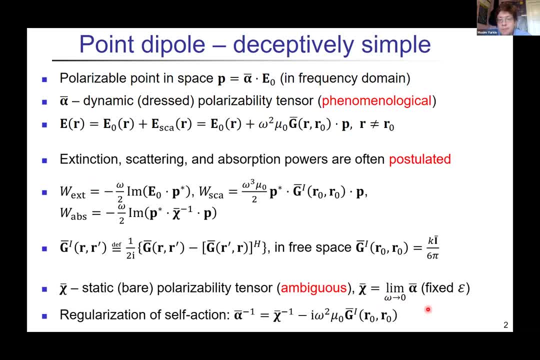 take this limit. One way to connect these two quantities is to assume some empirical definition for like self-action of the dipole in itself. I mean, if you take it just bluntly it will be singular, right, But you can take some regularization, for example again using this GI term, and then 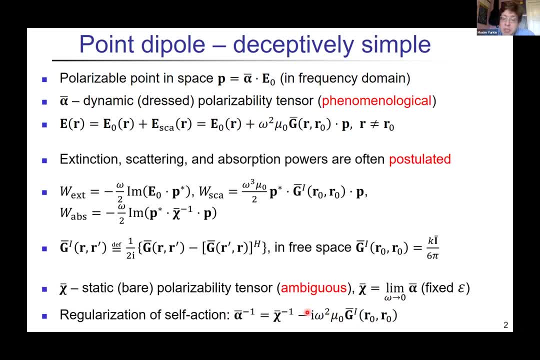 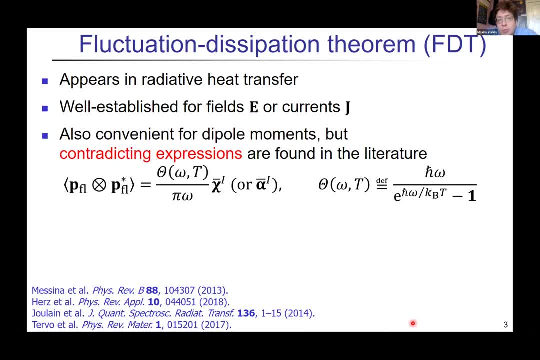 there is one of the possible expression that appear in the literature for connecting static and dynamic plausibilities. So that's part of the confusion. But when we go to fluctuation, dissipation theorem, which is well, something probably you never need, but if you want to consider something, 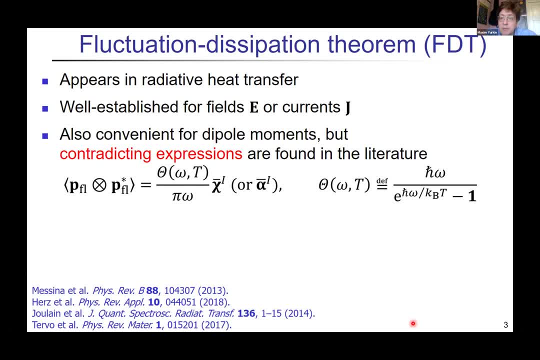 like radiative heat transfer, Cosmere forces, then it's very convenient. So you can compute some quantum quantities in terms of classical exodynamics, And this theorem is really well established for fields or currents. So there is no problem with that. But for a dipole 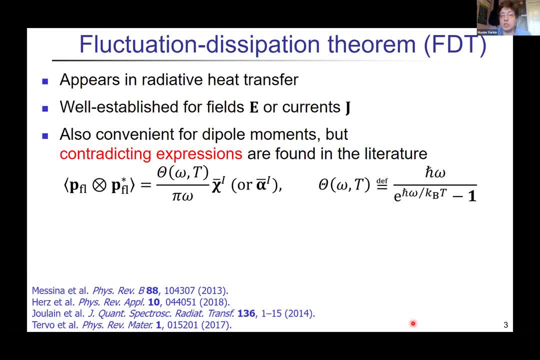 or a system of point dipole. it's convenient to write it down in terms of fluctuating dipole moments, immediate, something like that, And again in the literature. well, here examples. you see different expressions And the problem is that you have either chi or alpha here. 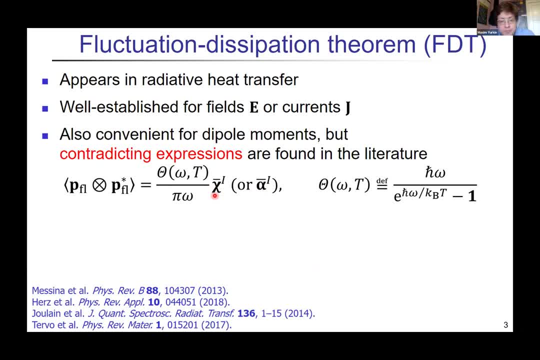 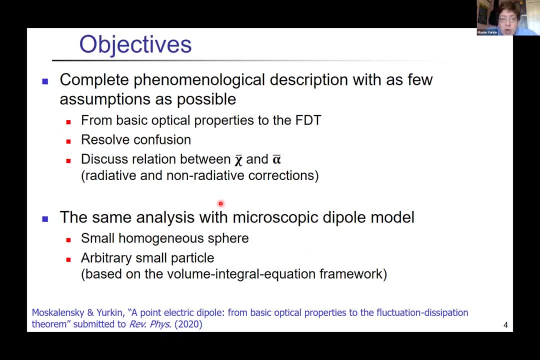 Okay, The difference can be actually quite significant, So that's a potential problem that we have here. So, given all these- I mean introduction- our objective was to build a complete phenomenological description with a few assumptions of possible, So to resolve some confusion and discuss relation. 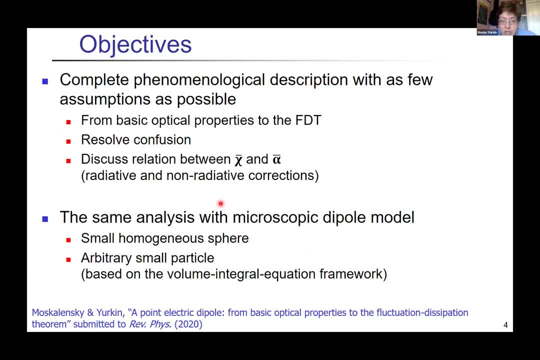 between chi and alpha, which is can also be related to concepts of radiative and non-radiative corrections of plausibility, which also often Are mentioned in the literature. But then we take also the next step and make the same analysis, but with microscopic dipole model, And here we use either a small homogenous sphere, 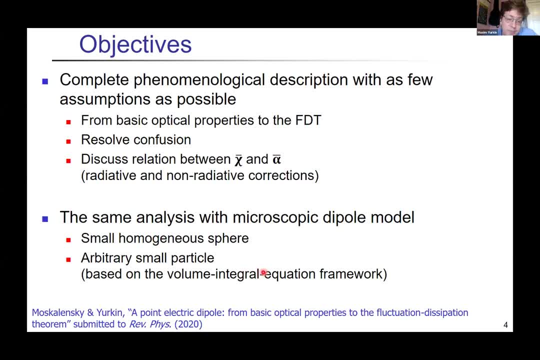 the simplest model or arbitrary small particles, And this part, well, in parts, is really new. So we basically did all derivation based on the volume integral equation framework And well, as you can see, there is really a lot about it And hopefully our paper will appear. 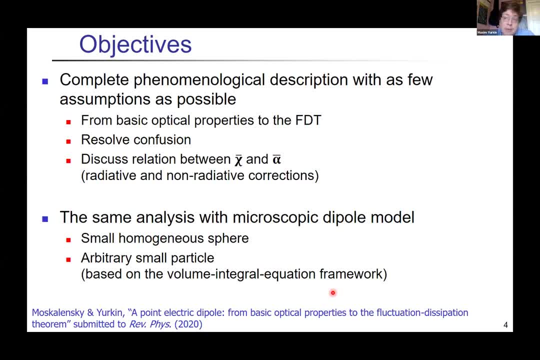 soon, which is kind of semi review paper, has a lot of math in it. Due to the limited time, I will only highlight some most important things in this talk, but feel free to ask me and I can send you the paper also if you're interested. 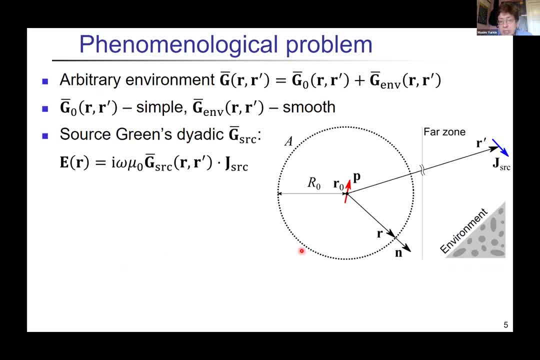 So first we discuss the phenomenological model. We start with the green stance, as I mentioned, which is a contribution from free space, and also some environment, possibly, And then we also use the source gains dyadic. That's exactly the one that 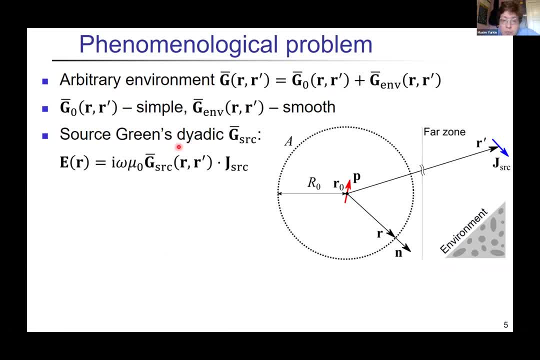 The previous speaker was also using. So that's something that connects every current placed in one space to the field in another point, which is induced both by environment and also by the dipole itself. So, basically, that's more or less a definition And our first result. 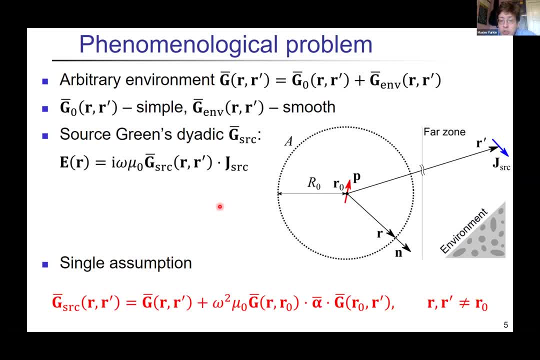 is that we show that you really need for a point dipole. you need only a single assumption to describe it phenomenologically Well, all of it's obvious. Yeah, So you need to define the source gains dyadic. Well, if you look at this equation, it's kind. 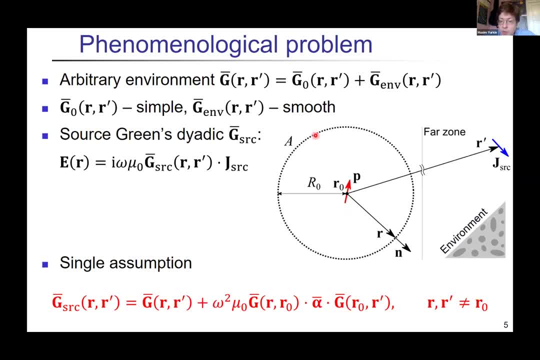 of natural. but once you do it, you can take, for example, a small sphere around the dipole which is much smaller than distance to environmental sources, and then integrate pointing vector around it And from this you can rigorously derive all the quantities which I mentioned. 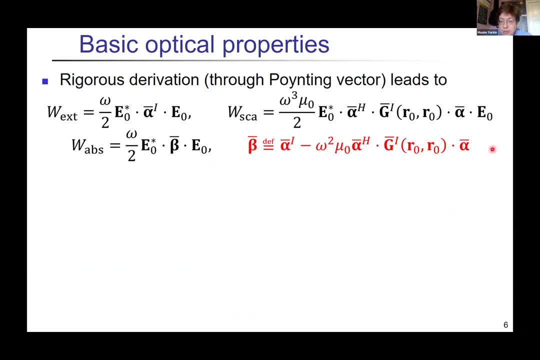 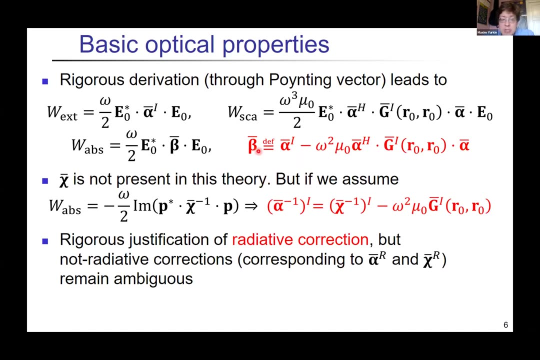 previously And here better is a convenient definition like that. It looks a bit complicated, but that's mostly because we use this, We use this general tensorial description, So if all everything is color, then it would be much simpler. Again, as I said previously, this description does not need a Chi at all because we have 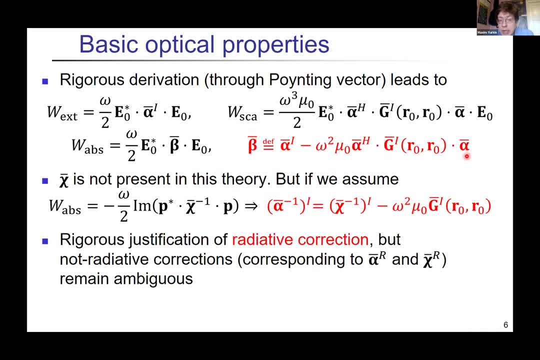 only a single definition, single assumption, and this assumption contains alpha as a phenomenological constant in it. But if we assume that absorption power is given by this equation, which is kind of logical because absorption is a local property, So it should be determined by the 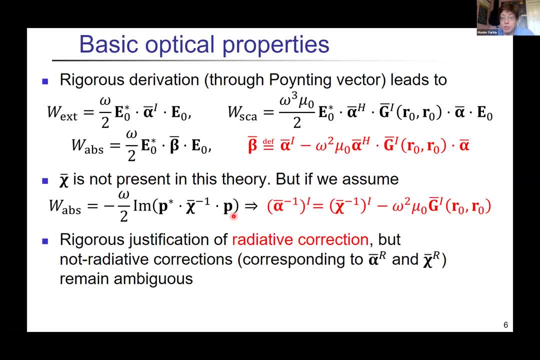 independent expression which is determined by something like internal fields inside the diaper, whatever it is. And then, if you assume this and just compare this to expression, we can actually derive the following relation between static and dynamic plausibility. Importantly, it relates: 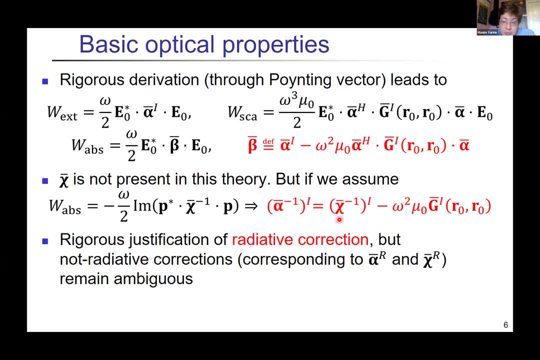 only the imaginary or skew-Hermitian parts of the plausibility. So that's actually justifies the radiative correction of the plausibility, but not radiative correction, Because non-radiative correction relates the real or Hermitian parts of this plausibility. So that's an example. 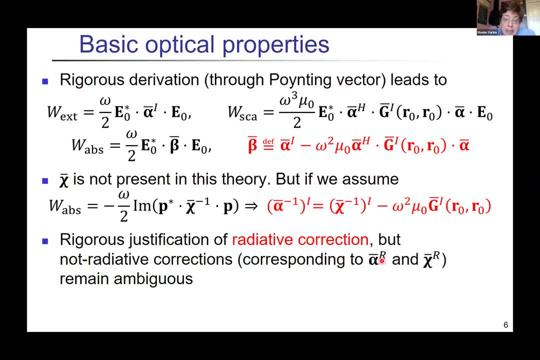 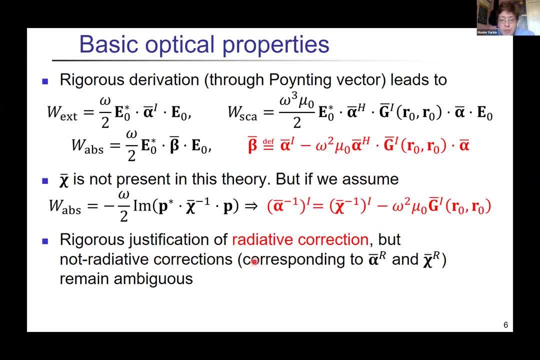 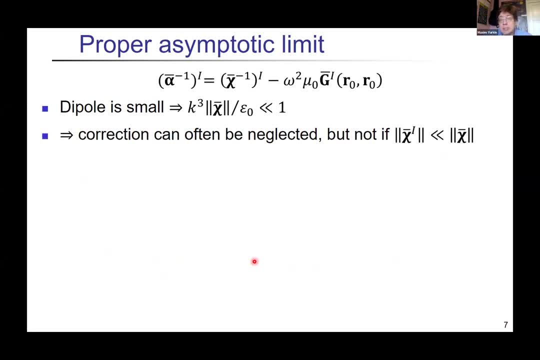 remain ambiguous and for a deeper discussion of this concept, we need to consider what is the proper asymptotic limit in this case. The problem is that whenever you consider a small dipole, you implicitly assume that it's small. yeah, obviously so, but when the dipole is small, actually its 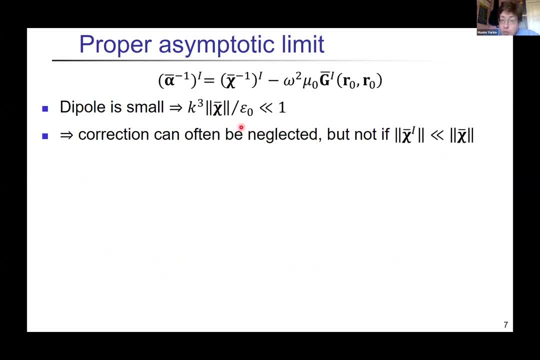 plausibility, as shown here, well normalized properly, is also small. so that's kind of implicit assumption that you have. and then if this is small, then those two should be large. so then you may think that, okay, we can always neglect this term and no correction is needed. 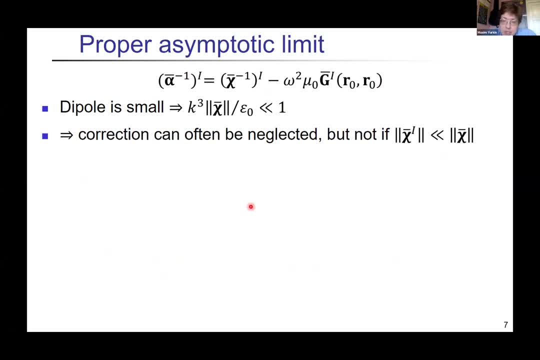 at all, and this in some cases true, but not if absorption is small. so if the imaginary part of chi is much smaller than chi itself, well, absolute values or some norm of the dyadic or absorption is not present, for example, then definitely you cannot neglect this term and this. 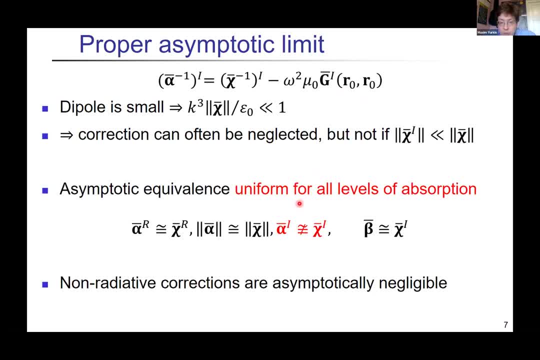 brings us to a proper understanding of asymptotic equivalence, which we will describe by this symbol. so we say that two quantities are asymptotically equivalent if they give, if they're like. well, in the limit they have the same small size limit, but this limit should be uniform for all levels of. 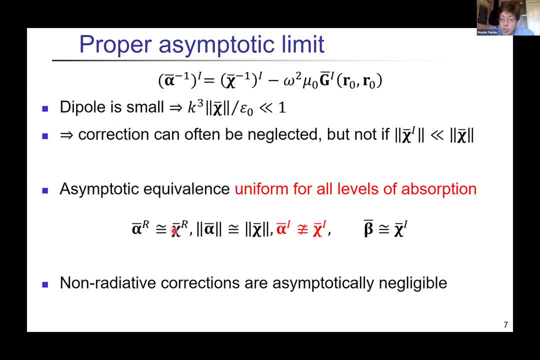 absorption. so in this sense the real parts are always asymptotically equivalent and, for example, beta is always a symptomically equivalent to a part of chi, but alpha and chi imagine parts of them. they are not asymptotically clueless. so, and that's justified that we should include radiative correction. so they're important for 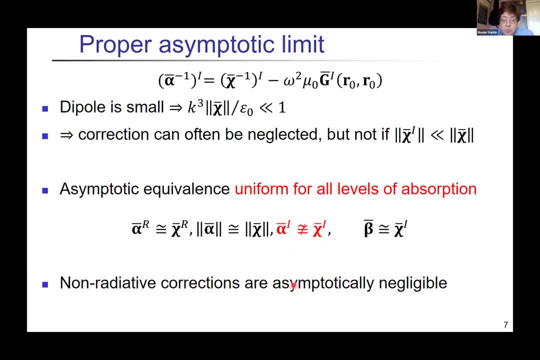 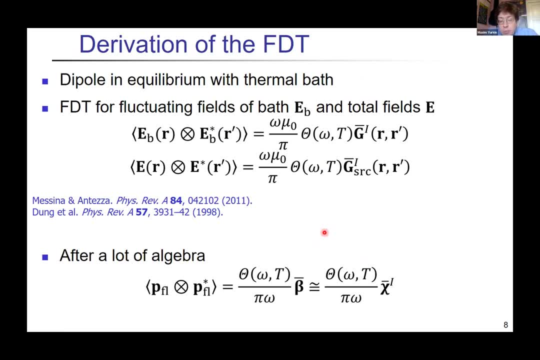 this asymptotic limit to hold, but non-radiative corrections, as i mentioned previously, they actually asymptotically negligible. ah and well, find. the final point of this phonological we've already discussed is that those elements should be potrzeb phonological theory that we can, again based on this single assumption of source, greens dyadic. 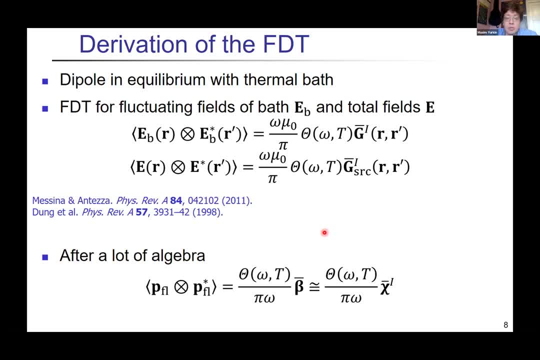 we can derive the fdt and for that we we do it in the most general setting of tensorial everything and basically we have it for for the fields. so the expression is uh. expression for the fields is given here. uh, it's either for fields in the bath or the for the total. 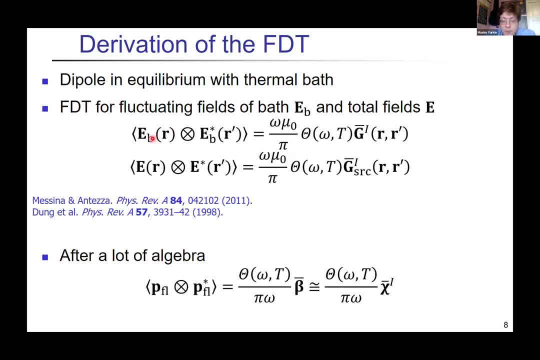 field. and then from this, after a lot of algebra, you derive the expression for fluctuating dipoles. so that's basically one of the expression that was used in the literature but disproves the other expression, and that's completely it goes. having said all these, uh, let us discuss really briefly. 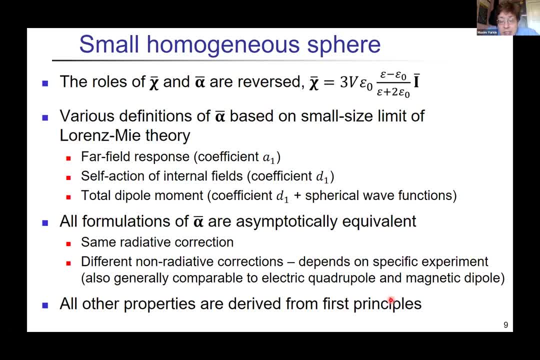 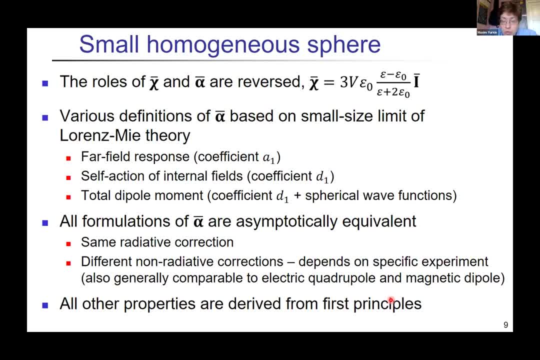 first important thing here that the roles of chi and alpha reversed, because everybody knows the electrostatic solution for a sphere and it gives us electrostatic possibilities. so no problem with that. we need only to know the dielectric function. here we have a uh scala expression. but it can be. 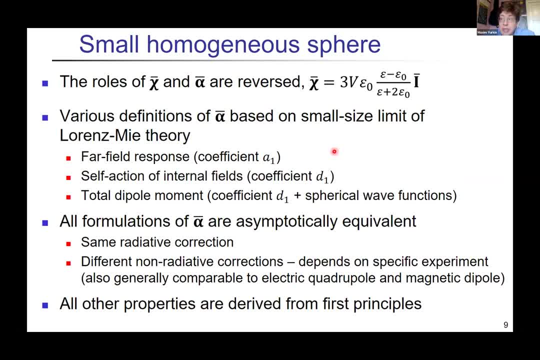 well, tensorial as well. uh. the problem is then that we have a law and smi solution to be able to lessen the uh. they begin to work and then again it solves us everything. but given this solution, it's not trivial to unambiguously define the possibility. at least, there are several options which are mentioned here. 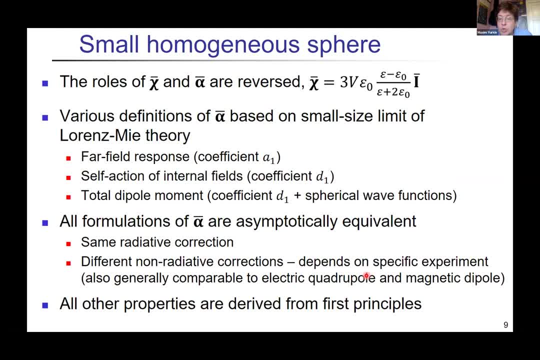 and all those formulations are actually statically equivalent and they also have same radiative proper choice, i think will depend on the specific experiment. so that's kind of a problem with them. and also another issue that if you look closely like on the total moment in the next correction it will depend not only on the incident field. 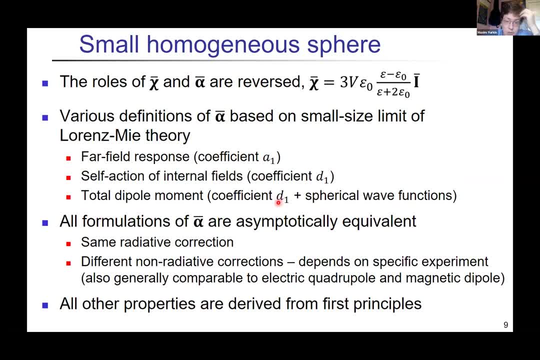 but also on the derivatives of the field. uh, there was a talk uh about it yesterday, i think. uh, so that's another issue which had some bigity here. but then, after we say this, we can also derive all other properties like absorption, whatever powers, and f and the fdt from the first principle, so we don't need any. 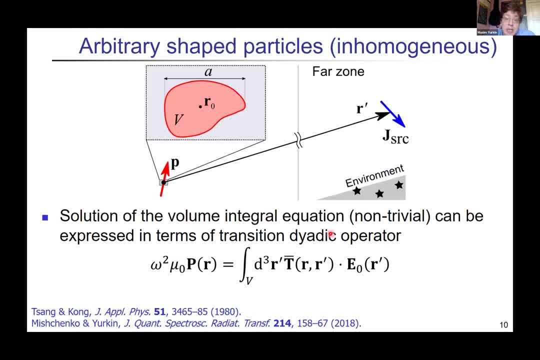 empirical assumptions here and the next step is to bring it all to arbitrary uh particles, uh, arbitrary shape, particle. and again the problem. well, it can be solved, but it's we're talking. you need to make some effort to solve the problem for a particle. here we write it down in terms of transition data. 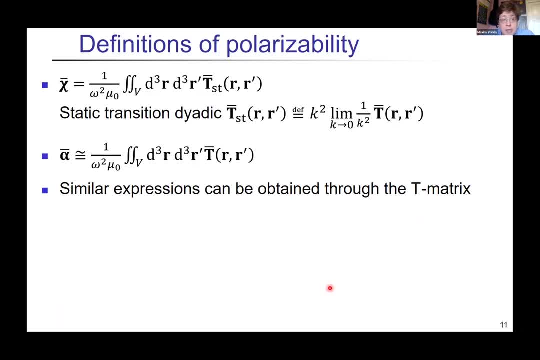 operators. so we assume it to be null and once we do it we can define anything we want. so, for example, the static possibility is given through the static operator and the dynamic possibilities given through the well standard dynamic uh solution at some fixed frequency. again, here you have asymptotic equivalent. so that's one of the possible definitions. 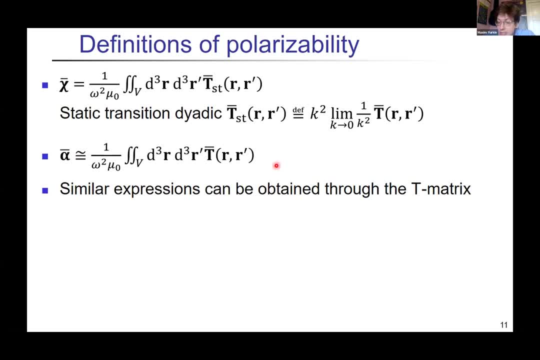 and well, if you are more fond of say which more or less the same operator, but in spherical wave function basis, then you can also do it. and one thing that we kind of accidentally uh obtained in all these uh regals expression is the expansion of inverse possibility in powers of a. 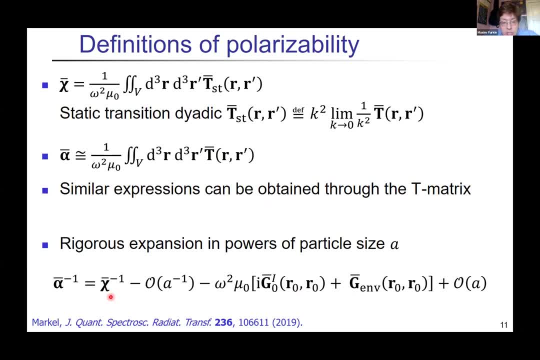 so it's shown here, and uh, so it starts from a to power minus three terms here, and then you have uh, the new correction, which is kind of complicated. but for uh- radiative correction- you have a uh, you have a clear expression. so that's kind of justifies the use of specific form of radiative correction. 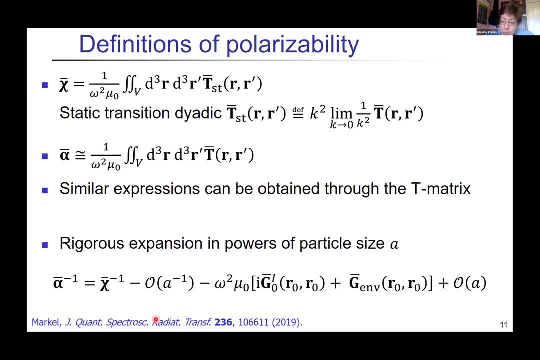 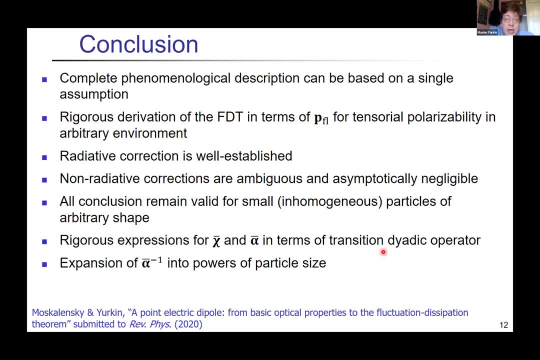 this was conjectured partly in the paper by wadi markel, but we proved it in a general setting. so that brings me to my conclusions. so first, while i argue that we built a complete phonological description that can be based on a single assumption, including the well, it gives us a rigorous duration of 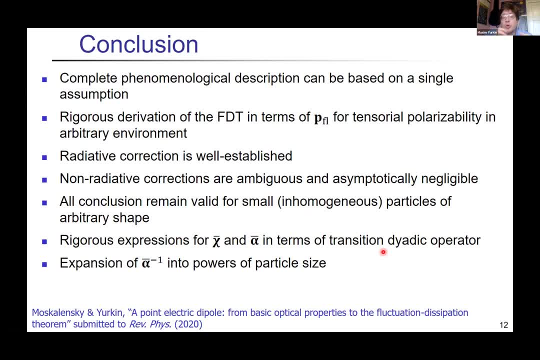 the fdt in most general setting. then we showed from all points of view that we considered: uh, the radiative correction is completely unambiguous and well established. by contrast, not radiative corrections are ambiguous and actually asymptotically negligible. so you really should try find a specific experimental setting where they would be. 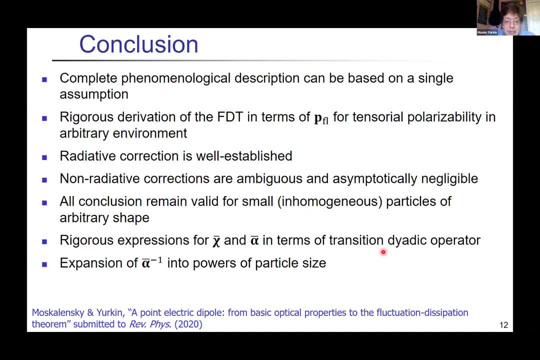 and all this conclusion, they remain valid for small homogeneous particles and also we showed the expansion of inverse plausibility into powers of particle size. so again i bring your attention to this paper, which have a lot of math and it kind of builds a complete framework for analysis of this problem. so if you 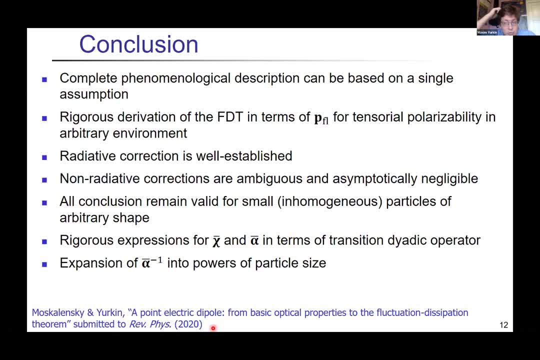 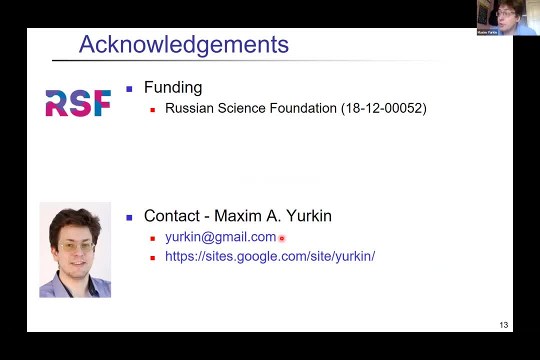 uh, want to do something- i mean the next step within it- then probably that would be useful, uh, for you. and finally, i thank russian science foundation for funding and thank you for your attention. thank you very much, maxim. so i think we have a question from hub. yeah, we have only one question, so 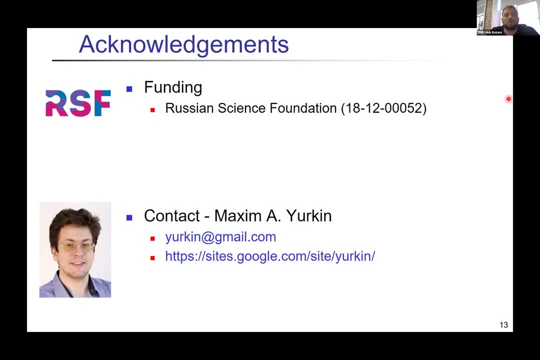 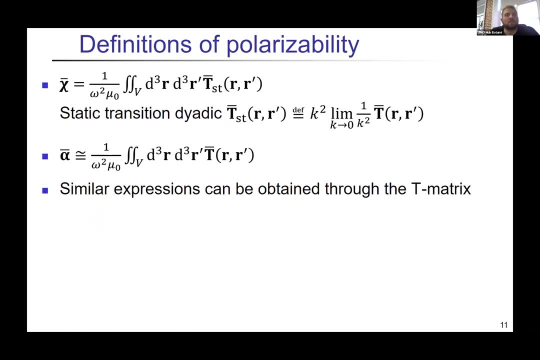 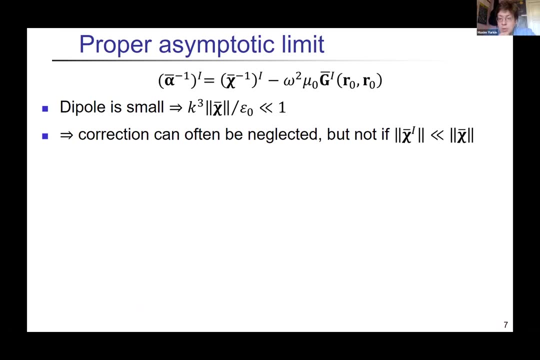 please, yeah, so very simple question. you defined your psi as something at the zero frequency. can you somehow adapt your formulas? uh, for dispersive materials can be put non-constant epsilon, epsilon which depends on the frequency. somehow at that, because this is probably which something which is interesting. 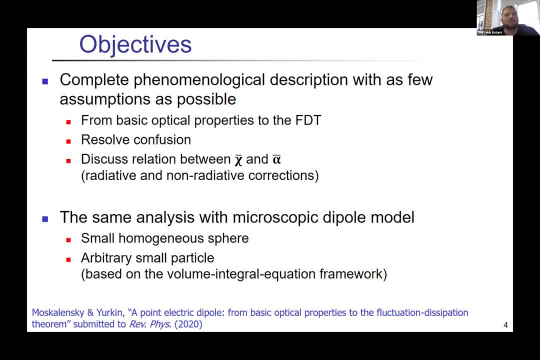 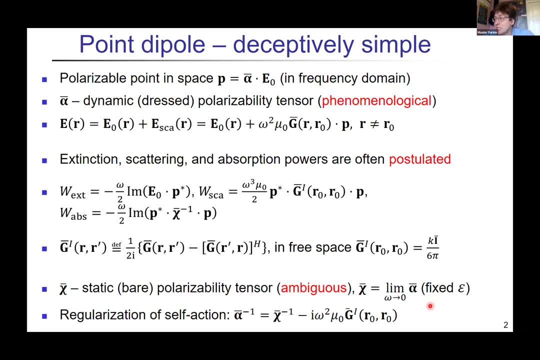 for uh, calculations of for real applications. yeah, yeah, that's exactly what i meant here. it's basically that everywhere when people use static, they actually mean that it's for a given epsilon. so you kind of want to take the limit of to zero frequency but keep epsilon fixed at some frequency, which is kind of of. 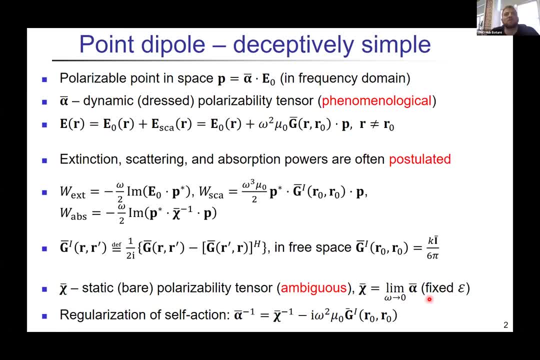 interest for you. so basically i can use just the ordinary formulas, just putting any arbitrary epsilon there. so i'm taking static of the there. so i'm taking static formula but placing i don't see take formula, but placing i would say seller for particular frequency and it. 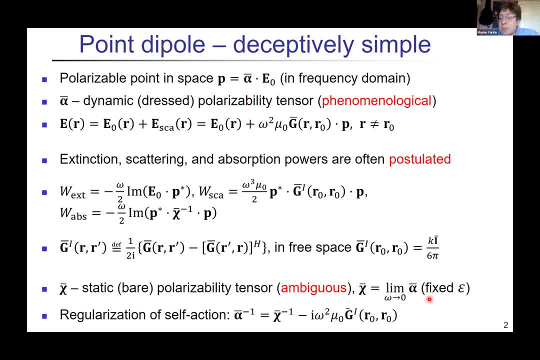 losses with everything. yes, yes, yes, have losses. lots will be some issues because of zero frequency, speptical losses. well, yeah, that's more less what you do, but i think your question more less highlights the confusion that is more or less highlights the confusion that is related to all, to all this issue. so